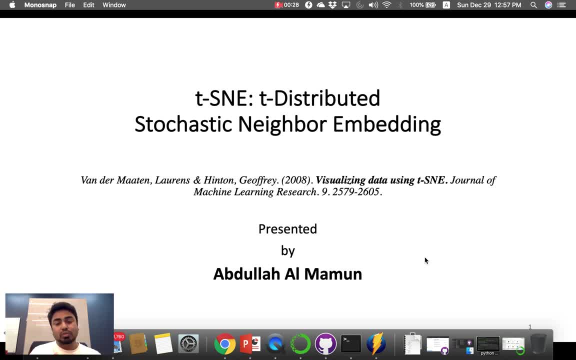 which machine learning algorithm you want to going to use So to visualize your high dimensional data set into a lower dimension. the TSNE is a right choice. So actually the TSNE actually developed by Mateen and Hinton, who is the pioneer of machine learning algorithms. So today I'm going to 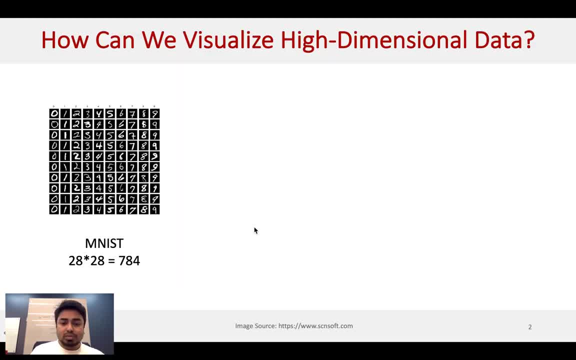 discuss about that. So let's move to the next slide. So, for example, the MNES data set, which is the handwritten data set of zero to nine, and it has 784 dimensions. So each pixel of this little image represents as a feature or dimension. So how we can represent this kind of 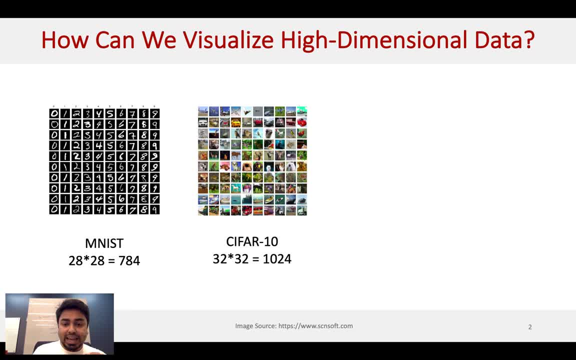 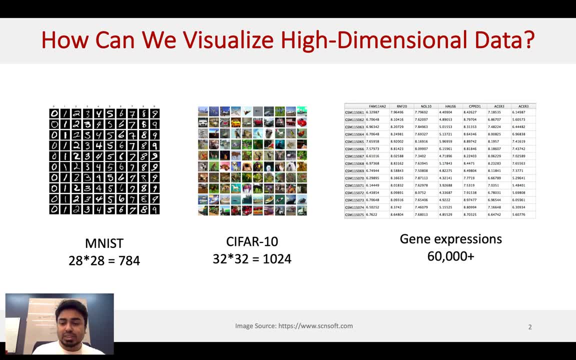 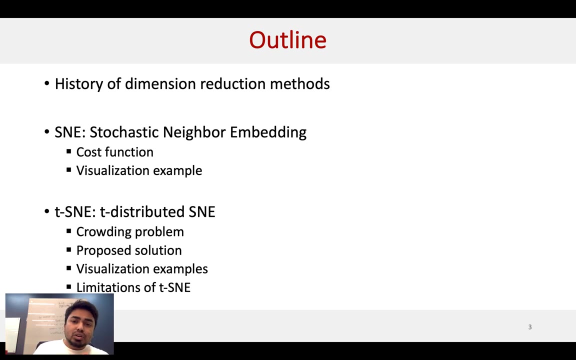 dataset And another one C for 10.. So there is a 10 color objects, so the dimension is 124, and similarly Xenix. it has more than 60,000 dimensions. so how we can visualize this kind of high dimensional data set? so we need a smart technique, for example TSA. so before 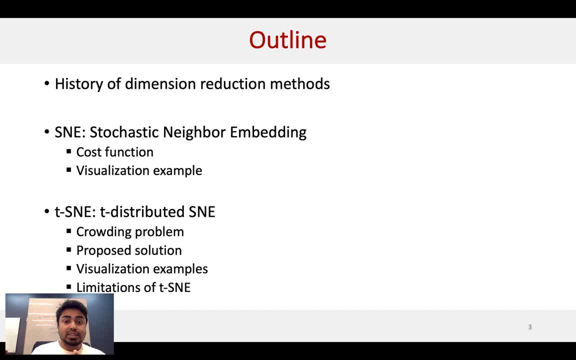 going to deep, we will see little history, because TSA is not a technique, is not a first technique. so TSA build upon on several techniques, for example the SNE, which is the mother technology of TSA, knee, which is abbreviated as a stochastic neighbor embedding. so we discuss about cost function of SME and 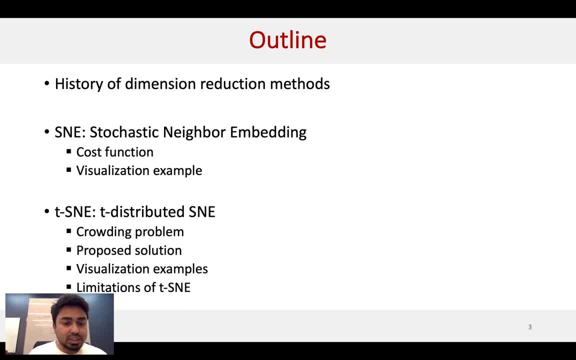 how some visualization example and of course, TSA need to distributed SNE. so what was the problem of the existing SNE is crowding problem. so we will talk about that and also how TSA need just this crowding problem in their updated version. see the visualization example and also the limitation of this. so the PCA is. 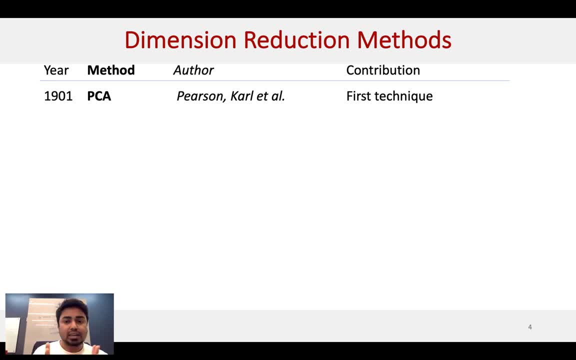 still popular method for dimension reduction. so this is the first technique which is proposed in early of the 19th century, and then isomers, which is the first nonlinear technique for data reduction, and then a scene which is the original SME algorithm proposed by Hinton in 2002, and then TSN e by 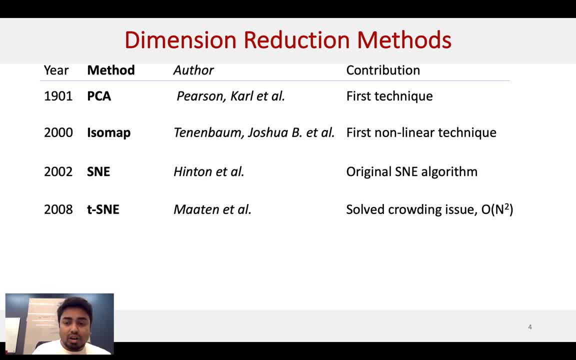 Mateen and Hinton. so it actually solved the crowding issue, but it has a severe problem of the complexity is very high, so it's there is a problem with performance. then they address this, they reduce the complexity, they improve it to n log n in 2014. but, however, we are going to discuss only SNE and TSN e. 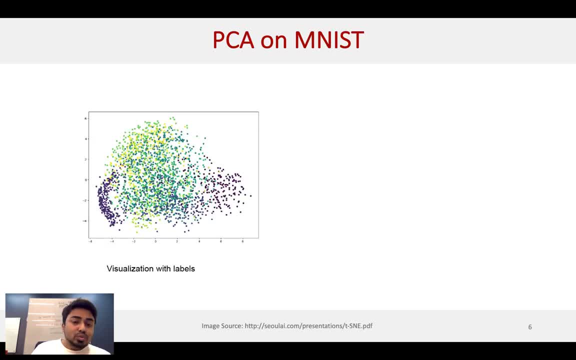 today. so if we want to visualize MNIST data set using PCA, the output or results will be exactly similar to this. so what is the problem? so we don't know the label. that means we don't know the 0 and 1 and 2, and which data represent which. 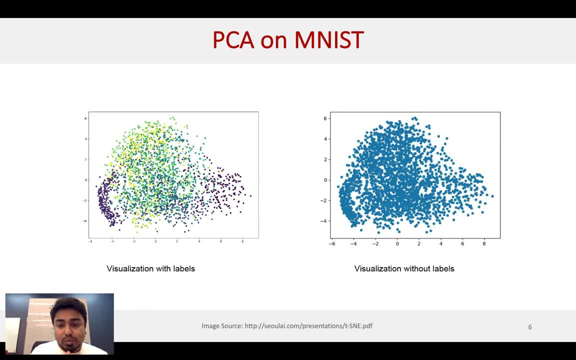 letter. so we don't know the label. that means we don't know the 0 and 1 and 2 and which data represent which letter or care or number without label information. so if I so, yeah, clearly this the color is showing each of the number. that's perfect. but if we don't know the, 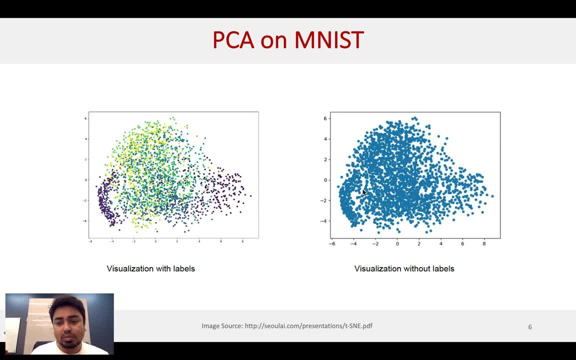 level, it will be looks like the second, all over the blue. there is no clear distinct cluster between 0 and 1 or the other numbers. so that's how we need a technique that can create the expectation is different, or 10 different clusters. right, so yeah, so why PCA fails to? 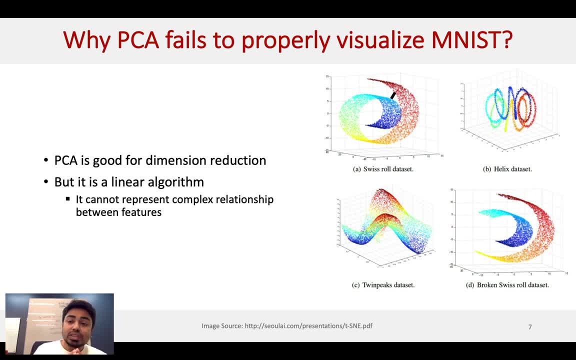 properly visualize MNIST because you know this is kind of non nonlinear, nonlinear data set, so PCA is linear. so PCA has big limitations when it's deal with the nonlinear data set. for example, if you see closely, look into the Swiss roll data set, so for example, the blue is a cluster. 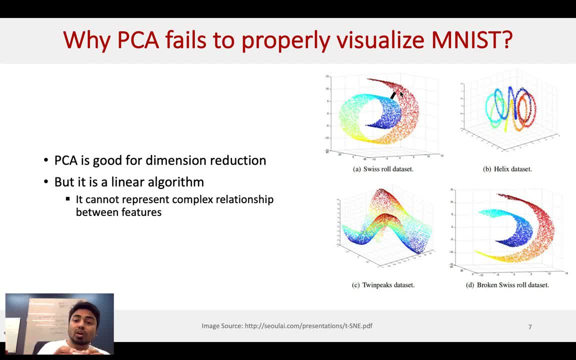 and rate is another cluster. so PCA works on the global distance. it doesn't look into the, into the clothes or the neighboring distance. that's the limitation. so here the distance is very small. so from red to blue distance is very small. that's why PCA will keep these two cluster together, because the 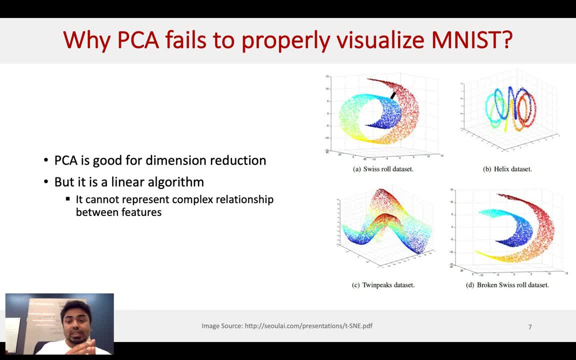 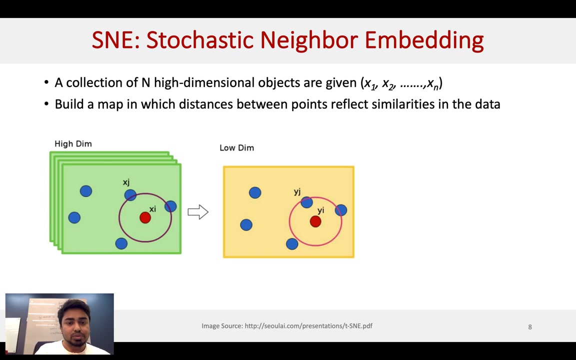 distance is small, so only PCA looks the bigger distance, so those are bigger. it will be bigger in the lower, lower space and similarly other other, some other database which are nonlinear and PCA doesn't work well for this kind of data set. so here S&E actually performing good. 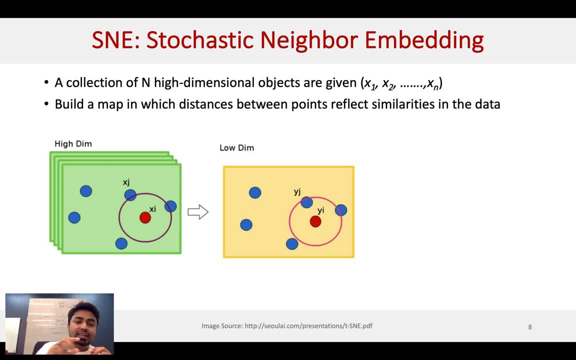 how? because they are working like here. if you see it's actually working. this is the high dimension, the green one represent the high dimension and in lower dimension we are kind of expecting the points will be on the same position in the same distance. that's how it's. 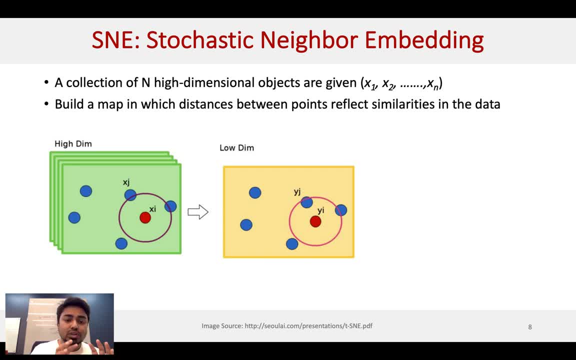 working right. so if we are, we want to keep similarity in lower dimension. how we can do that? so we have to measure the distance between two neighboring nodes and then we'll keep those distance similar in the lower dimension. for example, X, I and XJ are two neighboring. so how we measure the neighboring? because they just 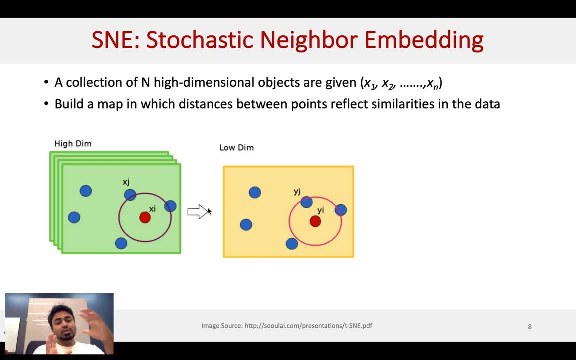 plot a Gaussian distribution curve. so those are those. those points are under the curve. they consider these are the neighbors of X- I. so then they actually kind of converting the distance between two neighboring nodes to a probability distributions. so build a map into his distance between points reflects. 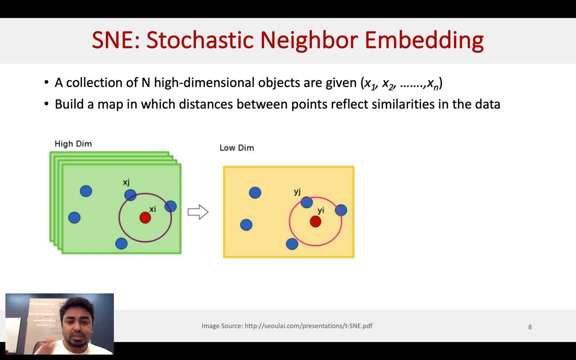 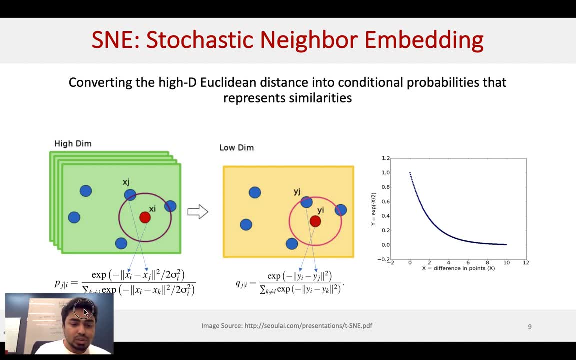 similarities in the data. data means the lower dimensions. so how? how they convert their distance to, to the, to the, to the probability? you see the, the Gaussian distribution, nothing but this equations. so if you closely look in the expression, exp of X, I minus X is so they are kind of calculating the distance, Euclidean distance, between two. 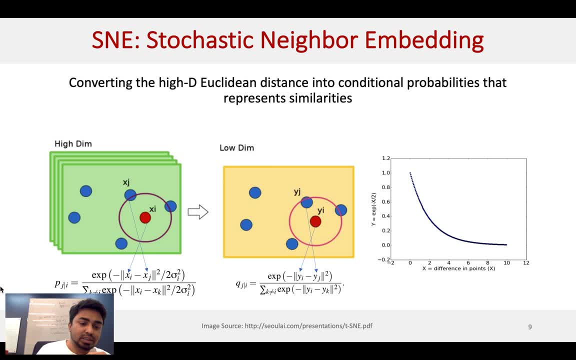 points and the they calculate the P J over I is so given I and similarly Q J I. so Q is the lower dimensional probability. so when these two probability are close enough that then we can say: well, these two points are similar between, similar in the height dimension and lower dimension. so yeah, so the right graph actually is. 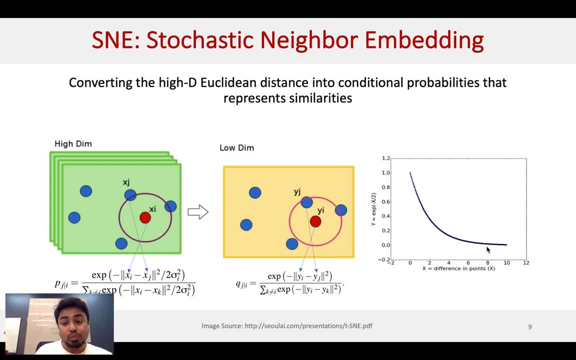 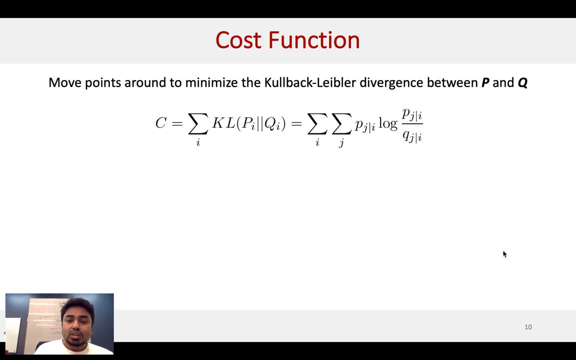 showing when the distance between two points is increasing at the same time the probability is decreasing. that means they will not be. they're not. most probably they will not be the same cluster because they are far well. so we need a cost function because we are minimizing these two probability. 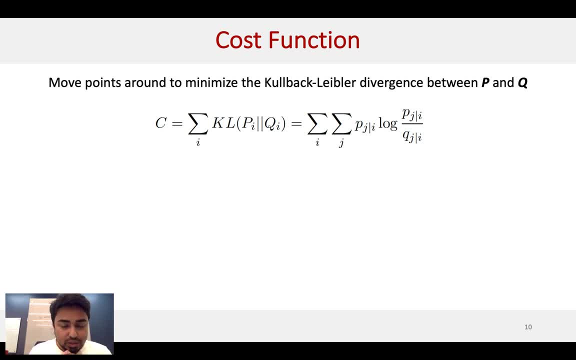 so the nice thing is why they could do they choose cool back labor diversions because of some nice properties, all of the nice properties. if P J I and Q J I is same, then this part will be. well, what would be this part? so this part will be one right and log on equal to zero. so the if the whole part. 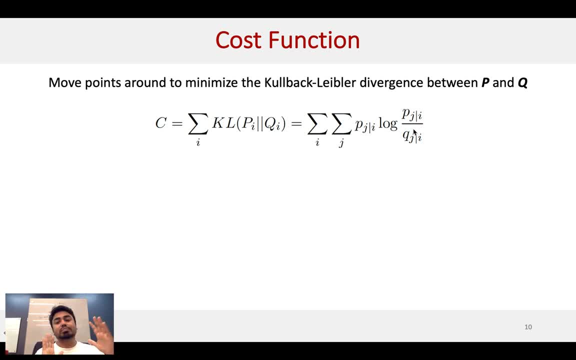 would be zero. there is no cost. if P, the probability in high dimension, and probably in low dimension, is same. well, the next next feature says so. it's kind of. it's kind of if, if P equal to Q, then it's fine, but if it's not, if it's not. 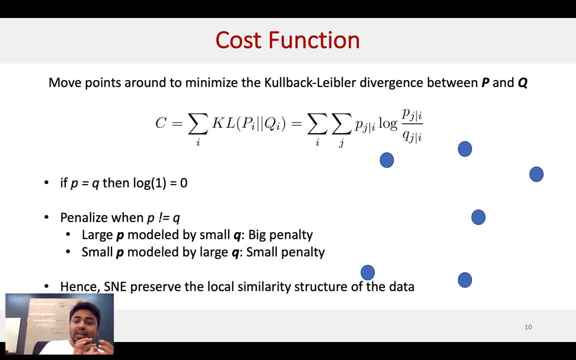 but this is not the real case. so we are that we are reducing dimension from higher dimension to lower dimension, so it will be not exact all the time. so if P is not equal Q, then there will be two situations: large P, large P or small P. large P means there is a big penalty because in, in, in higher dimensional, the 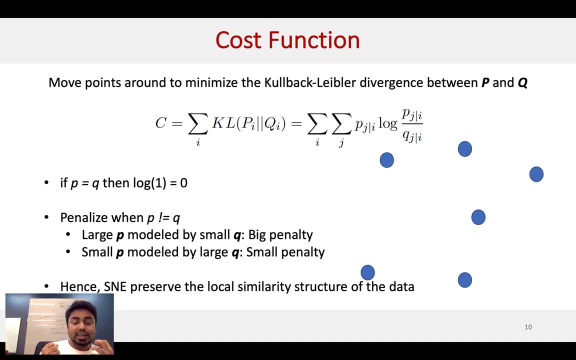 probability and the lower dimension will be higher than the lower dimension and the probability is not same. so large P. so that means we have to pay big penalty. but if, if a small P model by large Q, then a small penalty, which is obvious, right? so initially data points are located like this, then they try to. they. 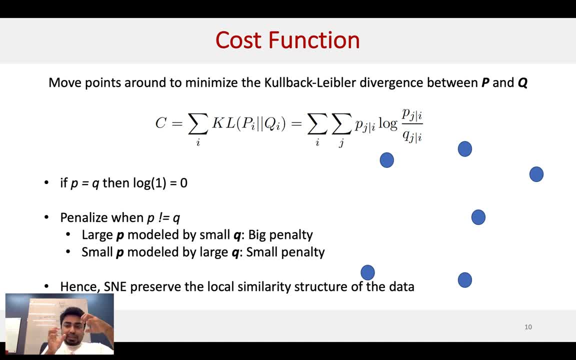 try to decide. this point will make make closer, or it will come closer, or it will be it will far apart. so that's how cost function is work. so initially, in lower dimension, the data data is data plotted in a scattered manner. then they calculate the cost function and those are needs to be come closer they come. 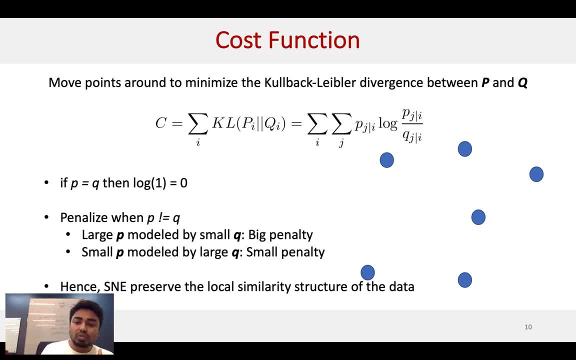 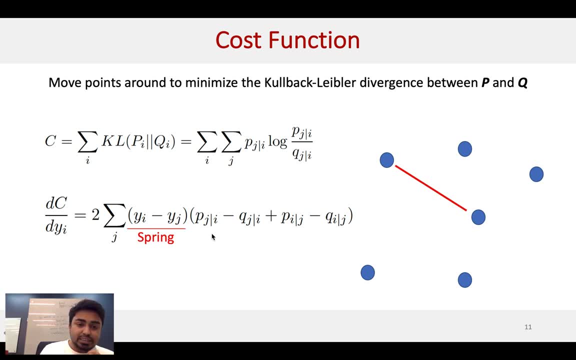 closer. those are needs to be far apart. they go more far. so yeah, so here for example: so this is the gradient descent of the given cost function, which is based on the cool back labor divergence. so if you see, if you see this part, yi and yc, the subtraction of these two points actually working as a spring. 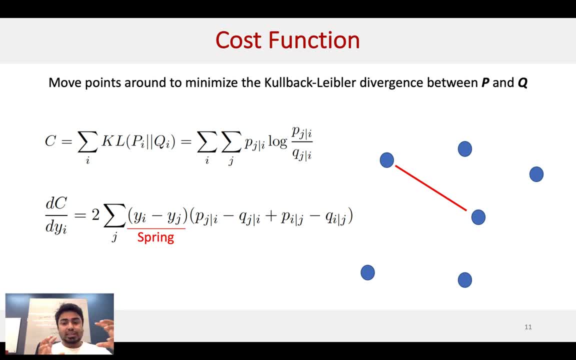 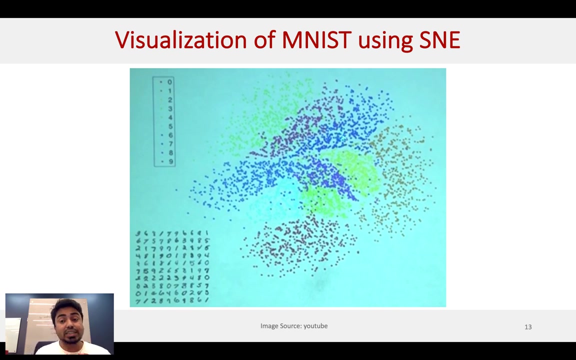 according to their paper. so again, these two point will come closer or it will go further. that's called extraction, so attraction or repulsion. so attraction or repulsion will be based on the second part of these equations. yeah, so if we visualize, you may miss data set using SME. we will see this curve. 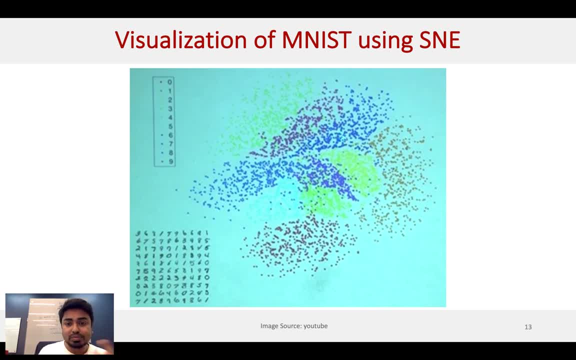 right, yes, yeah, it's. it's improved a lot over PCI, right? you can now, at least you can- see the different cluster right: the blue or green one and then the brown one. sorry for this figure, because I collected from YouTube and that's why it's not clear. so, yeah, so. so the thing that I want to show you is that, if you 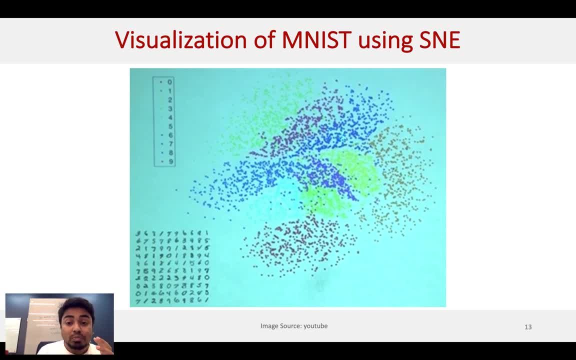 take a look at the graph, you can see that there is a little bit of a difference between the two points. so the thing is, there is some problem is still there, which is called crowding problem. you know what? you know what is the crowding problem? the crowding problem is if you look close into the center, there is 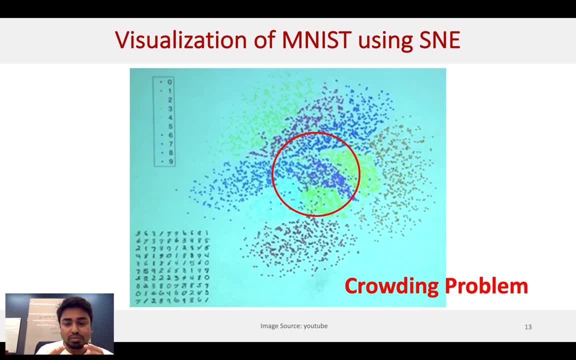 still some overlapping. so this overlapping actually actually gives some problem, which is crowding problem. so crap, it is space and we are trying to feed a lot of people in a small space. that's why crowding happens. so in in dimensional reduction technique, we have very limited space in lower dimension and we are trying to fix feed a lot of. 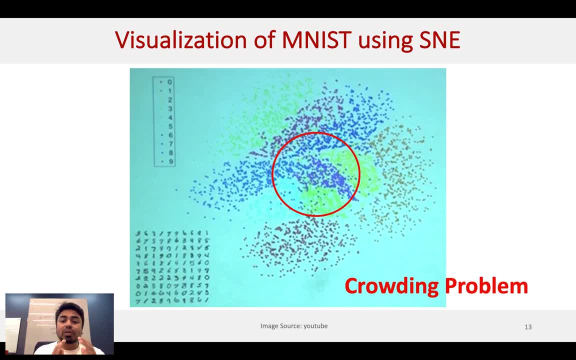 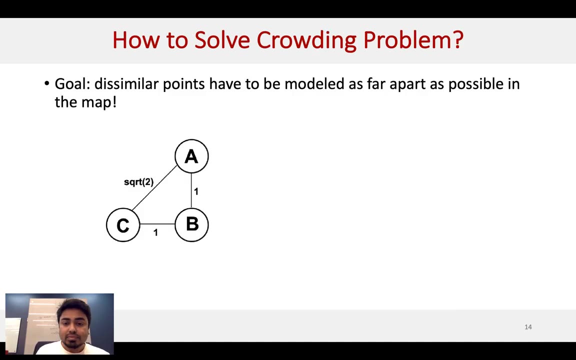 data points from the high dimension. that's why some overlapping is still there. so we have to overcome this crowding issue. that's how TSN comes and they address this crowding issue. let's see how they overcome these, these things. so yeah, so the goal is to 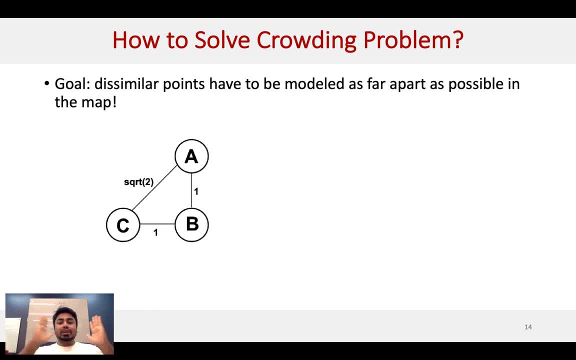 dissimilar points have to be model as far apart as possible. so the thing is that those points are located at the boundary of the Gaussian curve. they are located on the boundary. but what about the other other clusters? so so the boundary points of other cluster, they are also located at the boundary. so there is some some overlapping. 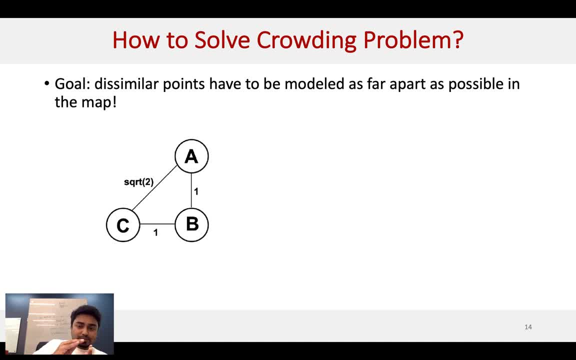 between two cluster or two type of data. so the the goal of tsn is to make the distinguish or make some gap between two clusters so that it will clearly, visually appealing, that that between each cluster, for example, how they do that. so if you see, we are now in two-dimensional and we are 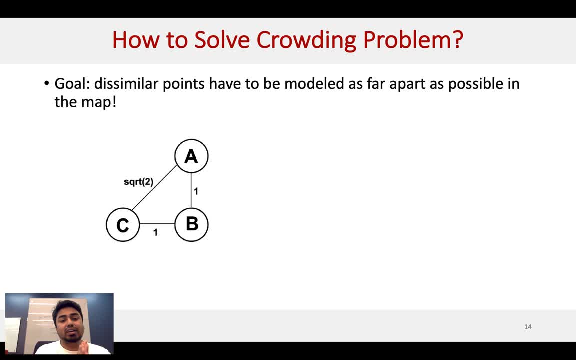 trying to convert from two-dimensional to one, and we so we cannot go beyond two-dimensional or three-dimensional. and so here, for example, we have three data points, so be to: a, the distance is one, and b, two or three, three points, one or two points is minus, and so, as you're going to see, we already discussed the, the flight data points, and here you will see the one area of the мира and air Shooter versus two chairs at key. Edit: Inica, b two cha chan and b twoüber is the area of the minha. yeah, how this case looks like. because we're so it is, it is little bit less difficult to actually. 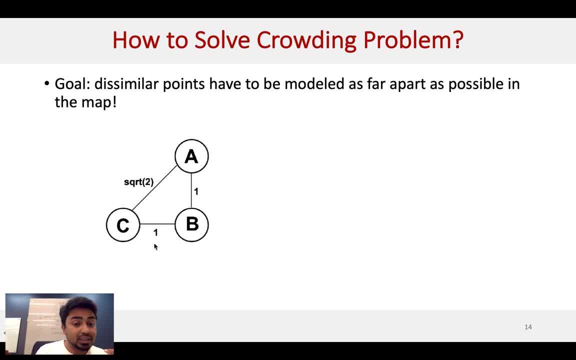 one butatifact to see if this case we will do some easyais use either. essentially it will. it is it's really difficult to call it simple order in here, because we meet that to see the distance is again one, but distance from A to C is not one more. 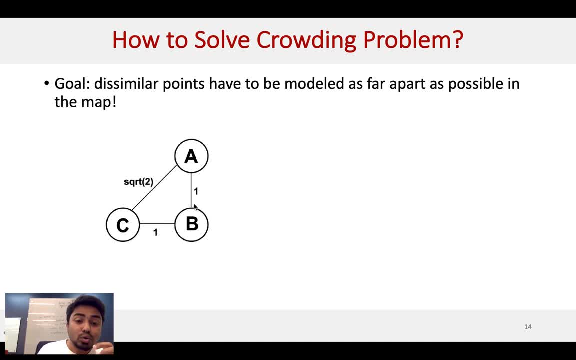 than one. so the theme is: those are the smaller distance, they will stay together, they will stay closer, but those are far apart. I mean, those are the distance between two points are larger, they will go even more far apart. so how? so if I put these two, two data points, from B to A and A to C, so if you see, we, we still 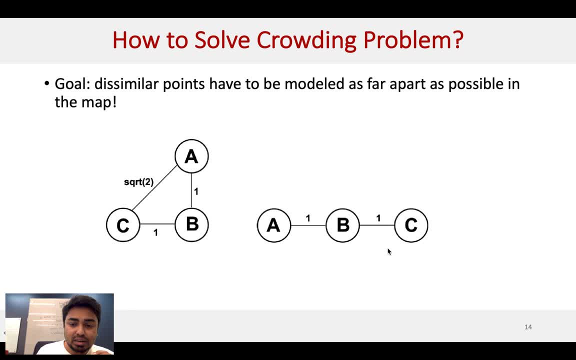 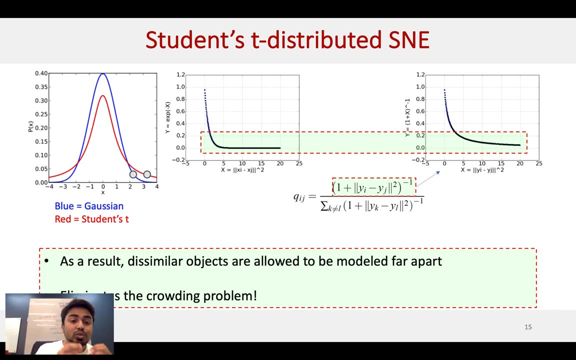 we? we keep them A and C closer, but we make A to C far apart, so that there will be small gap between two cluster, right? so so the what is the mean contribution? this is the theory, but what is the map behind this? so they just replace this. 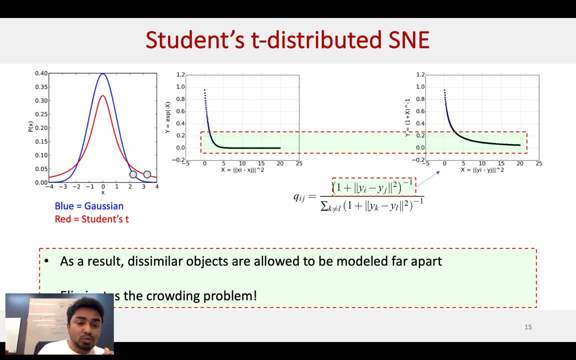 probability distribution curve. before it was the blue one, the Gaussian, now they use student t distribution probability. so that means what is the difference between these two? if you see, if you see the, the Gaussian, so at the lower probability, these two points, at the lower probability, at this distance, the probability for these two points are: 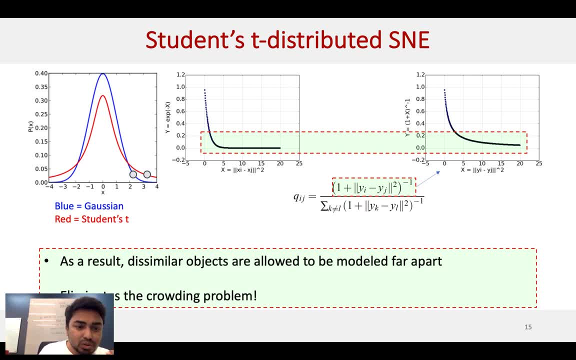 same right, which is which is little bit more than 0.0. so that means the lower probability means that this is greater than 0.0? I do not think it is. they should stay far apart. right, they should not stay closely because the probability is very low. but what is the difference? at the same probability, the 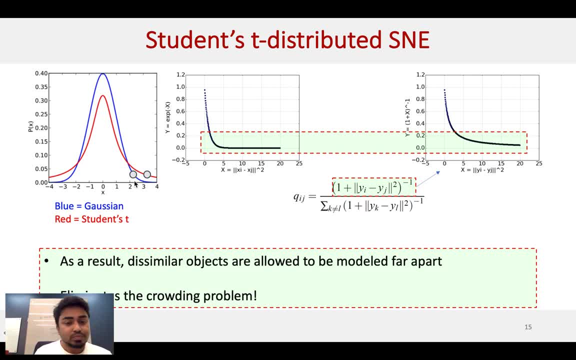 distance in Gaussian is small and distance in in in student is very large. that means there is a small gap. I mean it could, it will be able to, to, to locate or to, to put the points far apart, even far apart on the lower dimensional space. so yeah, so since the probability distribution equation has 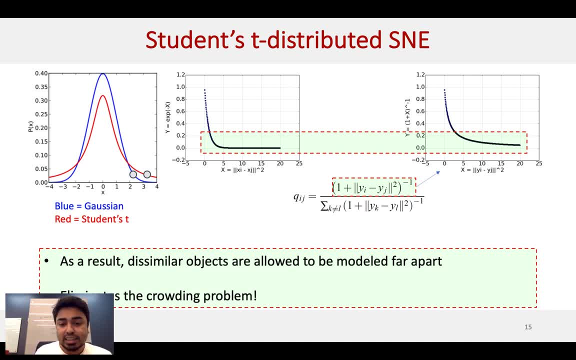 changed. that's why they change in the Qij, only Qij, remember, only Qij. in the lower dimension, not in the high dimension. higher dimension is still Gaussian probability distribution. in the lower dimension, which is qiz, they are calculating the student distribution probability, that's. 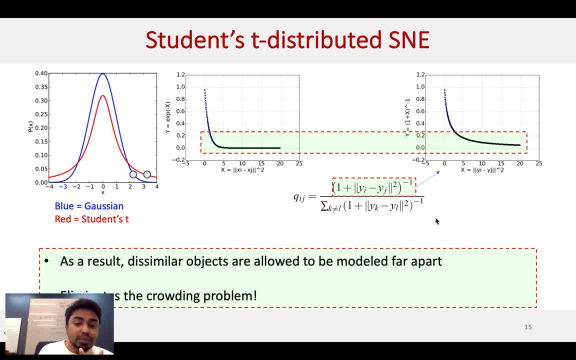 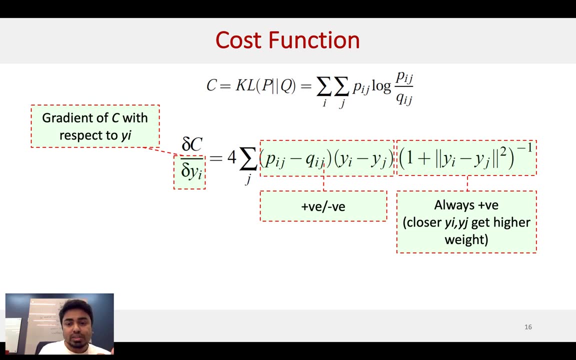 why the equation has changed. so, as a result, this similar object are allowed to be modeled far apart, and this is how they address the crowding issue. so, yeah, this is the new cost divergence equations. so here, the this part will be positive or negative, but this part, this part, will be always positive because 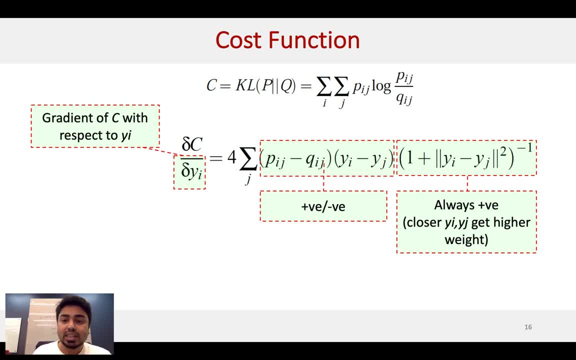 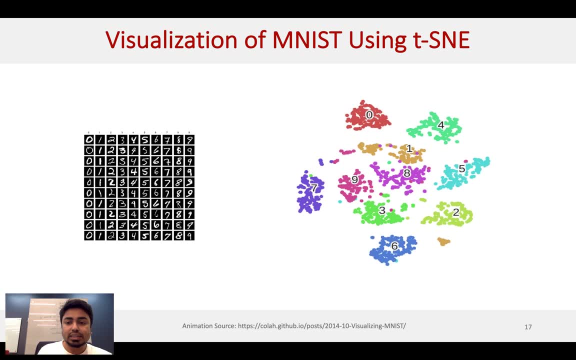 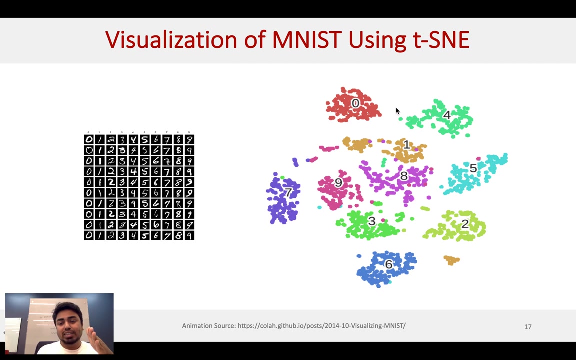 closer yi, closer yj get higher weight. so yeah, so now if we use visualization of MNIST, using TSNE, the data plot will be more like like this: so here, if you closely see on the, the plotting, so the gap between two clusters is more visually. visually, i mean if you see that the gap between zero and four is more right. so 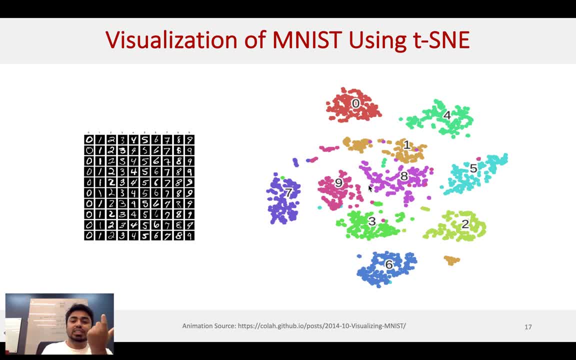 before it was like kind of overlapping. so if you see the student distribution curve, that example exactly is applied here. so the between two clusters, the gap, it increased. so this is their contribution. they said even the dimension of the data is very high but it is still evil. 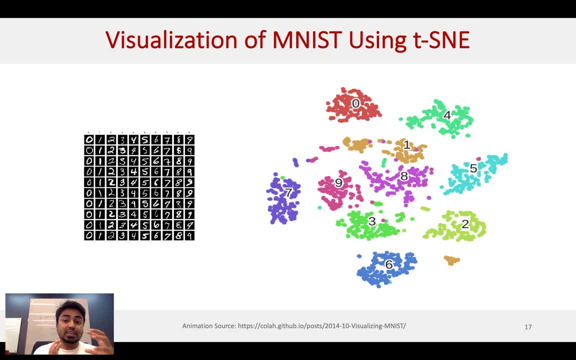 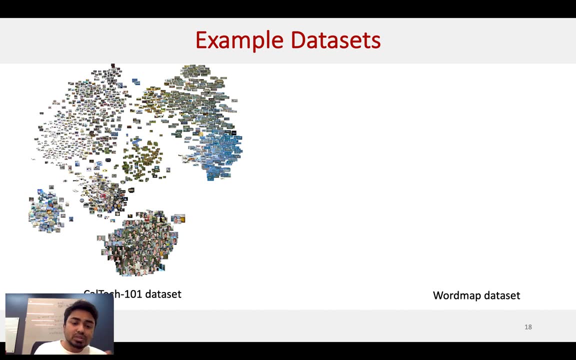 to create some cluster so that you can see how many cluster exist on your data set or how it looks like before training any machine learning model. so yeah, we will see some more examples. so is there's Caltech 101 data set, which has 101 different objects and you see the the cluster is clearly distinguishable. 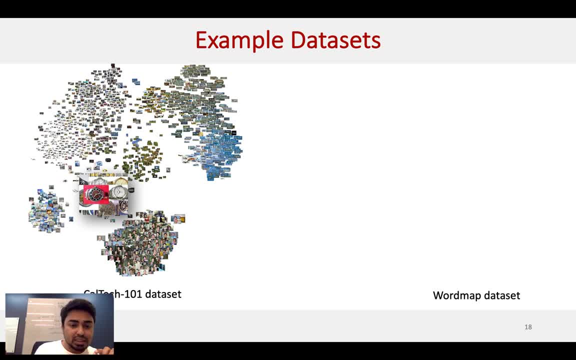 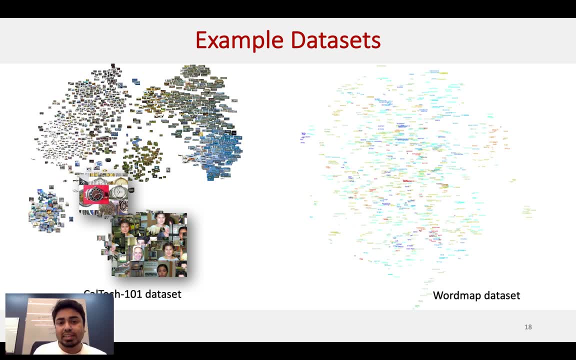 so, for example, this one is the image of hand, wrist was and then another one is human faces. so on the right hand side the data set, which is called ward map data set. so those word meaning are more similar, though we located on the on the same cluster, for example, here if you see died, crash, murder, and then another one. 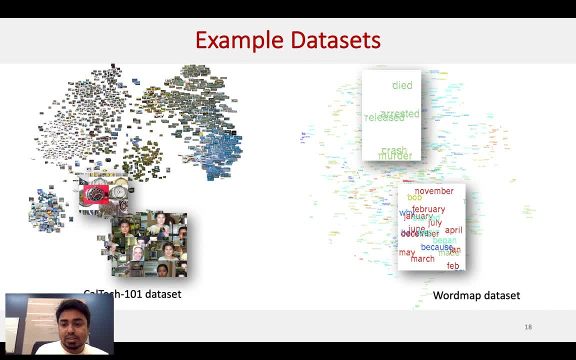 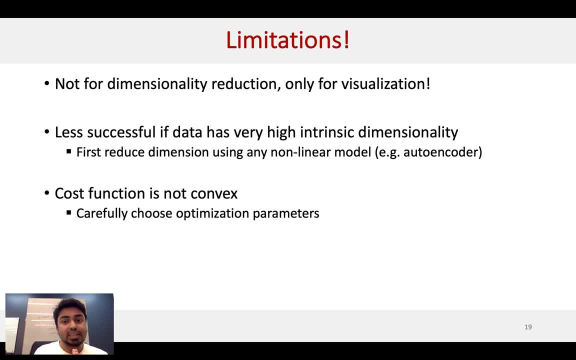 the 12 12 months, the name of the 12 months. so yeah, so TSN is best for visualizing any kind of data, but it has limitation. so the first warning is: this is not for dimensionality reduction. this is only for visualization. so you can use it for visualize the data, but not for reduction. 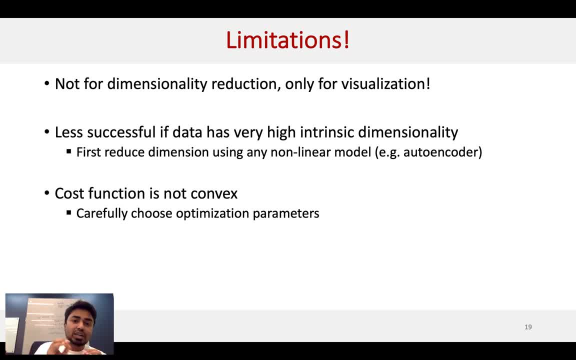 which is cannot do. reduction is only up to two or three dimension and less successful if data has very high intrinsic dimensionality. what does it mean? if you have really high intensity dimensionality, then you can use it for visualization of the data sets, but also for other non-linear ans, more than 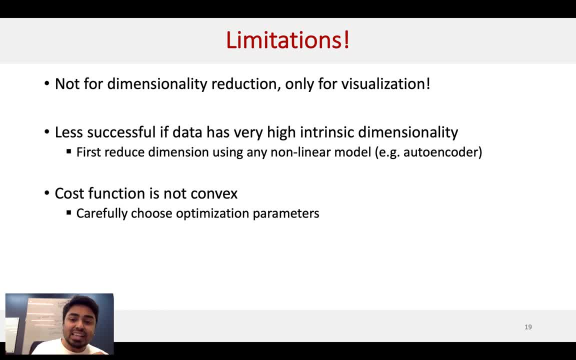 60,000 dimension. so if it is has really high dimension, then not go first with t-series before running in the running with t-series, first reduce the dimension using any other nonlinear technique like autoencoder. then use the TSN a because TSN the cost of teasing is very high, which is n square if you really 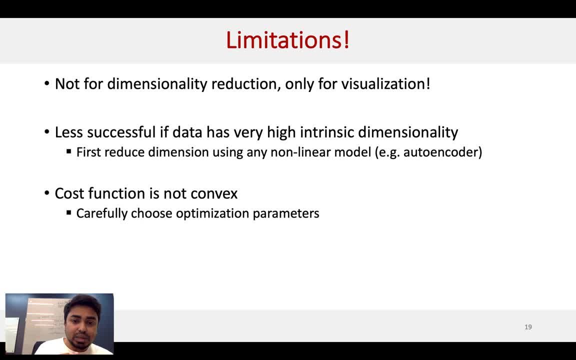 try. if you really reduce some dimension before using kcd, that would be, that would be cost effective, as cost function is not convex. so if you carefully, if you see there is some optimizing parameter, so for example, perfect city, then variables. so so you have to carefully choose. 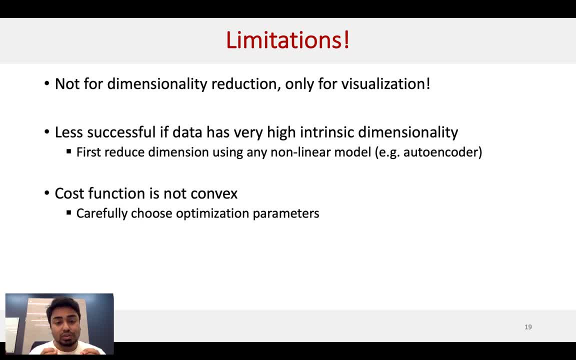 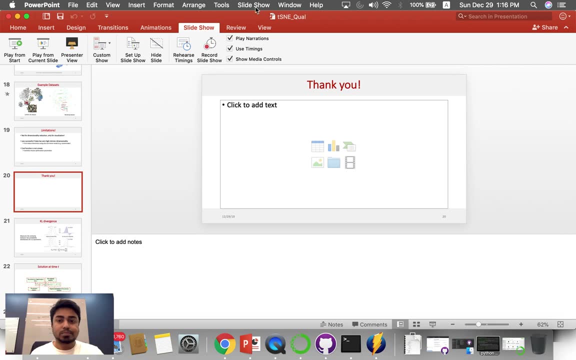 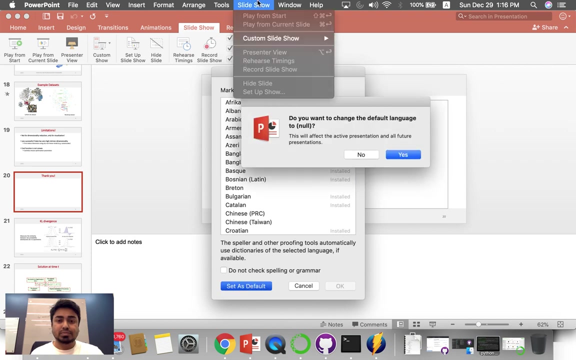 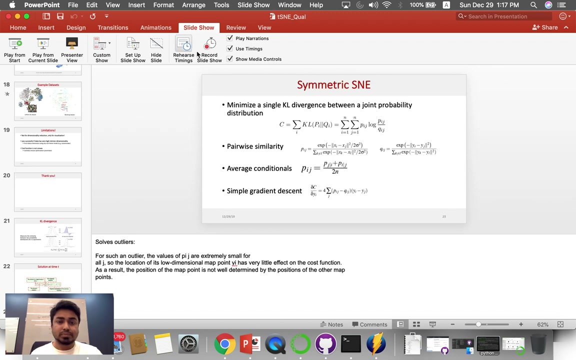 the optimization parameter. otherwise, if you, if you doesn't choose the parameter carefully, then the visualization would be different. it can be different. yeah, thank you. thank you very much you. 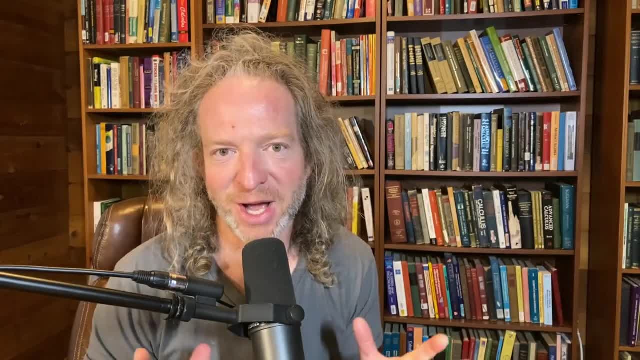 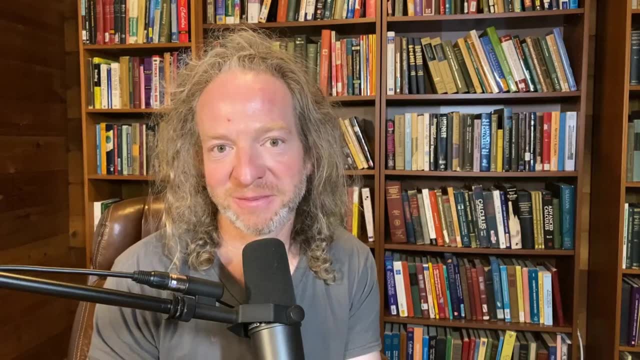 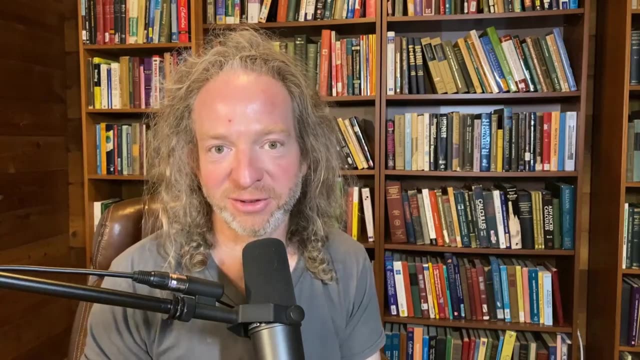 When I was in grad school I had to undergo these observations. Basically, what that means is a professor comes in and watches you teach And I was terrified. I was so scared. This was my first time ever being in front of college students teaching mathematics. It was basic calculus. 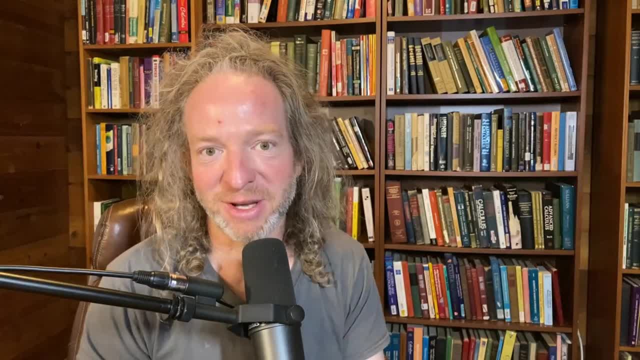 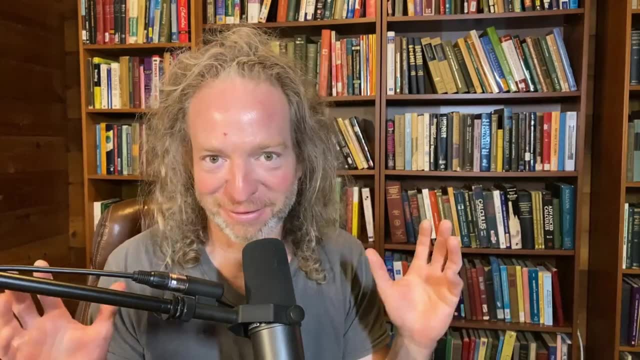 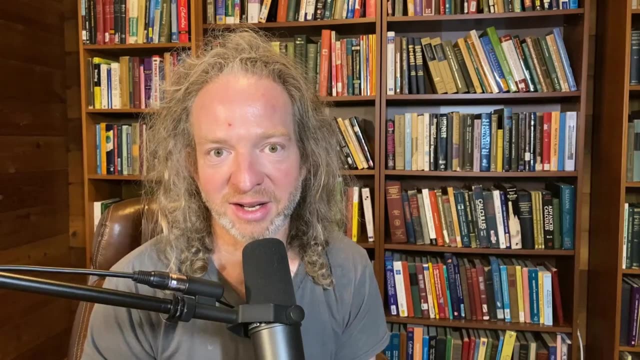 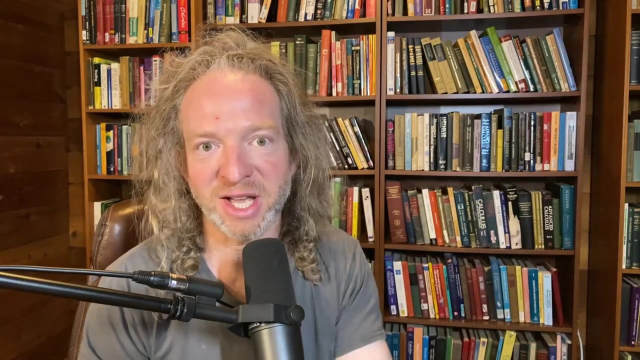 that I was teaching them And this professor came in and he observed me. Afterwards I met with him to you know, discuss the results of my observation And I had so much respect for this guy- and I still do- And he told me that I reminded him of him. He said: you remind me a lot of myself when I 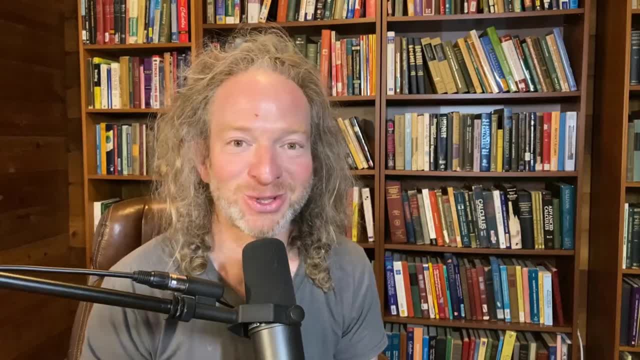 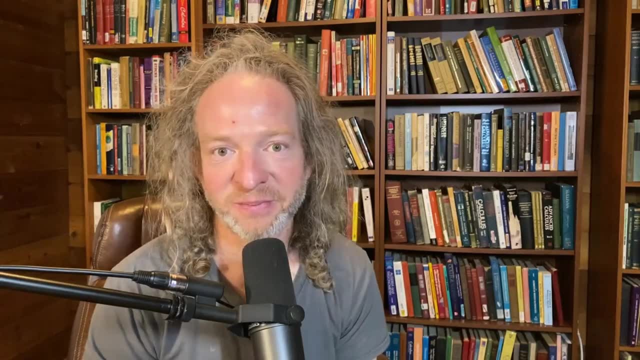 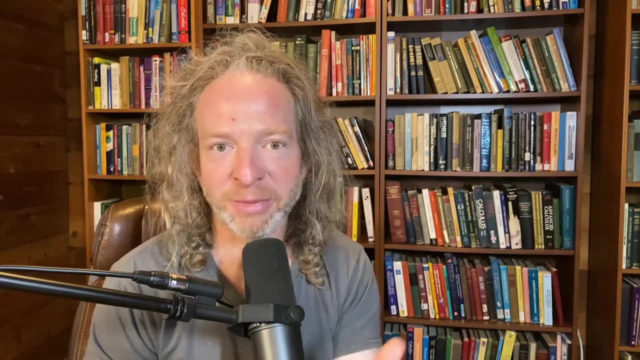 started. You're a lot like me And I was like, wow, this is really cool, because this guy had a PhD from Princeton And I just thought he was just such a cool professor, a great guy. He was never my teacher, but I remember feeling really good when he said that. So today I opened my email. 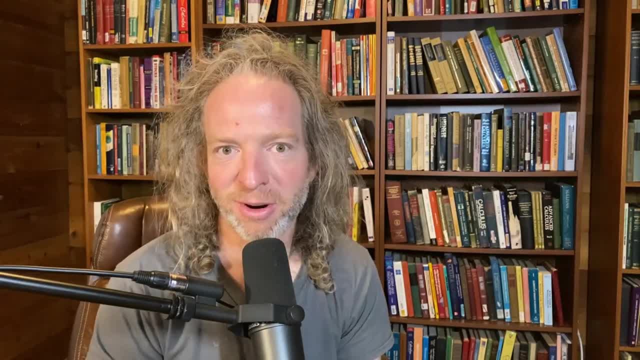 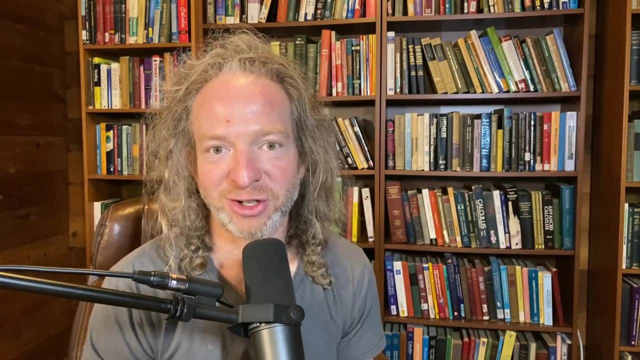 and I got an email from this guy. His name is Omar And his email reminds me of myself when I was starting college. When I started college, I was a high school dropout. I took a class in high school. I took a class in high school. I took a class in high school.